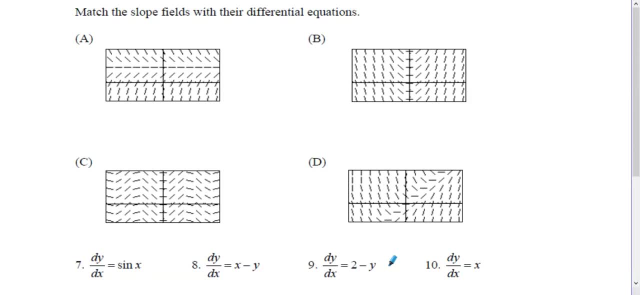 So my personal preference here is to look at where I have slopes that stand out Um. the slopes that stand out most frequently within a slope field or within the differential equation are going to be the places where the slope is zero. Like you can probably look at slope field A here and pretty clearly realize that right across. 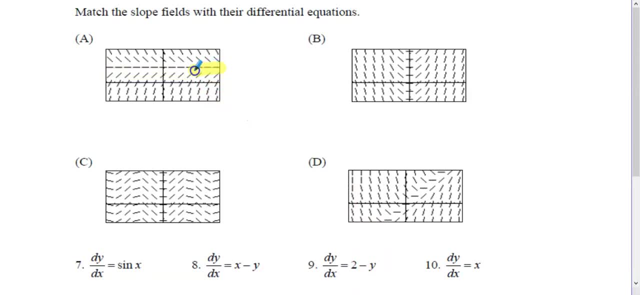 which was difficult for me to highlight. let me try that again. right across this horizontal, we have a sequence of zero sloped segments. So what's true about all of those locations where I just highlighted? Well, x is definitely changing because I'm moving back and forth across the graph when I 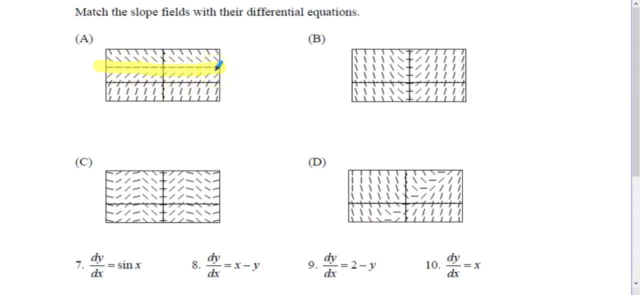 pass from this straight side of the graph to this side of the graph, But what's not changing is the y value. I'm not moving up or down at all. Looking at a y value of zero on the x axis and a y value of one across this diagonal. 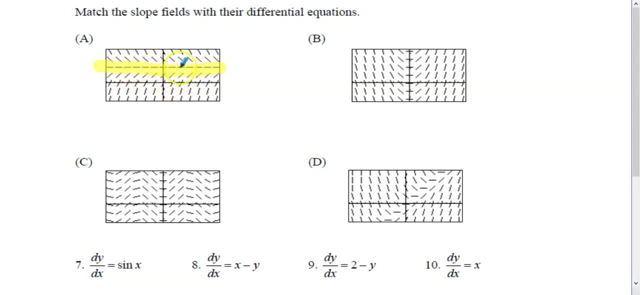 or across this horizontal. excuse me, then, this horizontal must be at a y value of two. So it seems like my slope has to be zero when y is equal to two. Look at your derivatives. Do any of these derivatives have that property of always being equal to zero when y is equal to two? 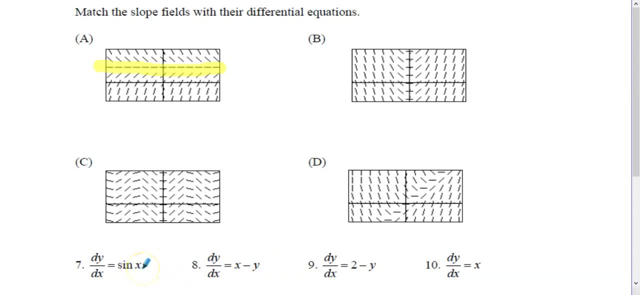 Well, this doesn't depend on y at all, so I can't really do anything with that. This depends on x and y. I might have to analyze that a little bit further. but then look at this one. If I put two in place of this y, 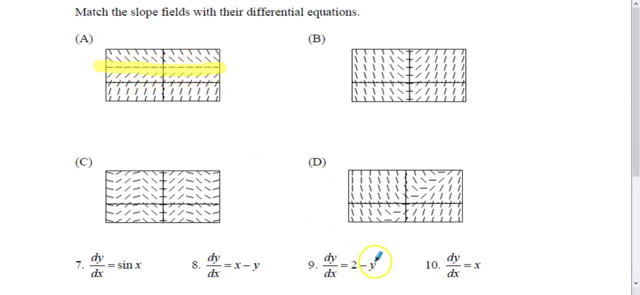 because that's where these zero slopes are. two minus two is zero, Regardless of what x is. this differential equation has a value of zero when y is equal to two And therefore, what we're going to be able to claim is: we're going to be able to claim that this slope field matches up with differential equation number nine. 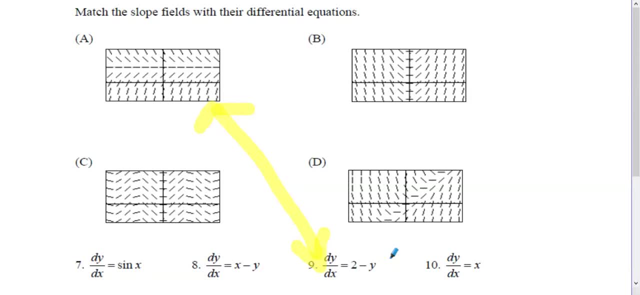 So we've got a matched up with nine. Let's move on to b. So if we look at slope field b, do you notice any places where you have zero slope? Well, in this case it looks like it's straight up and down the 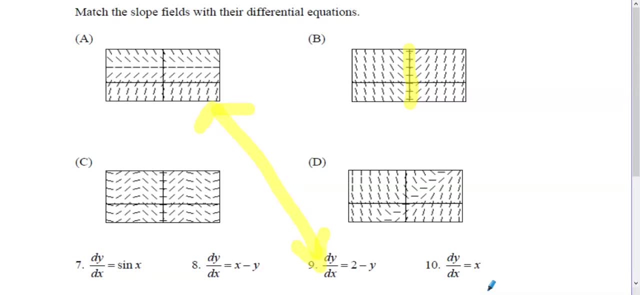 y-axis. What's true about all those points on the y-axis? All of those points on the y-axis have an x value of zero. Do any of my derivatives, do any of my differential equations have that property of being equal to zero is equal to zero. 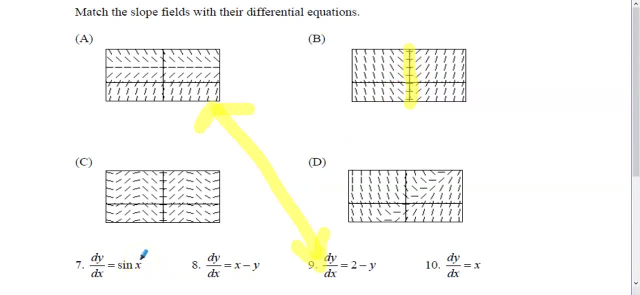 So if you look at number seven, sine of zero, Well, sine of zero is zero, so this has that property. This one here depends on x and y. so, like we kind of said about choice a when we were trying to match it up a minute ago, 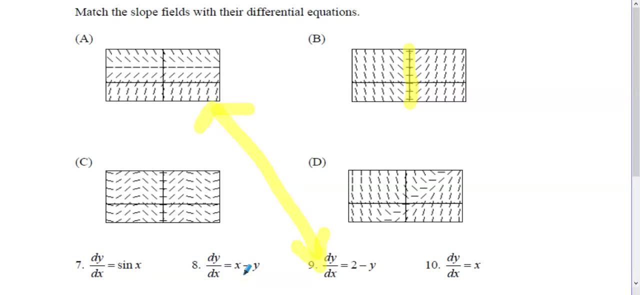 That one we might have to analyze further, but we'll see if we can narrow it down with, without getting too involved with that. first This one: well, yeah, when x is equal to zero, this one's equal to zero. So it looks like we have two differential equations that have the potential to match up with this slope field. 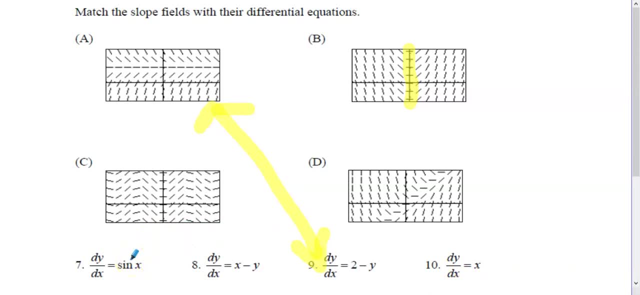 because two differential equations have the property of being equal to zero when x is zero. So now we have to look at other information. So the rest of the information that I like to look at is typically going to involve the sine, not the s-i-n, not this sine. 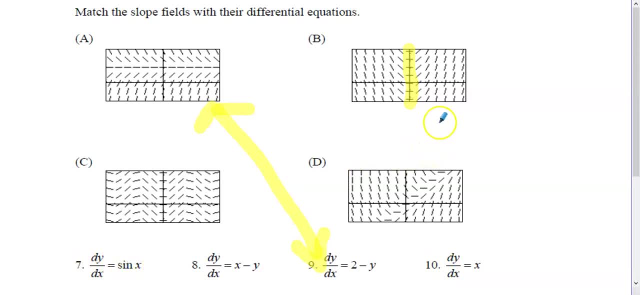 but s-i-g-n of my line segments. So I see that in my first quadrant here for this slope field, my slope is positive. In my first quadrant x is positive. Does this have that property? Is this derivative going to be positive when x is positive? 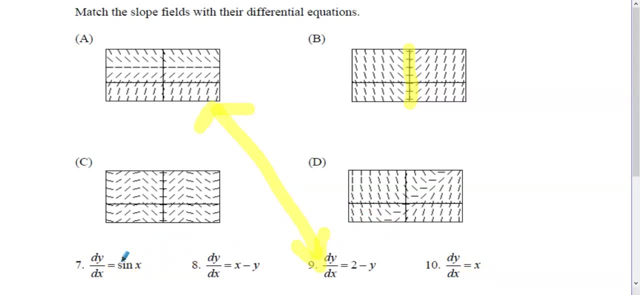 Yeah for sure Does this have that property. Well, sine of pi by 2,, that's a positive number. Sine of pi by 2 is positive 1.. But 3 pi by 2?? 3 pi by 2 is also a positive number, and the sine of 3 pi by 2 is negative 1.. 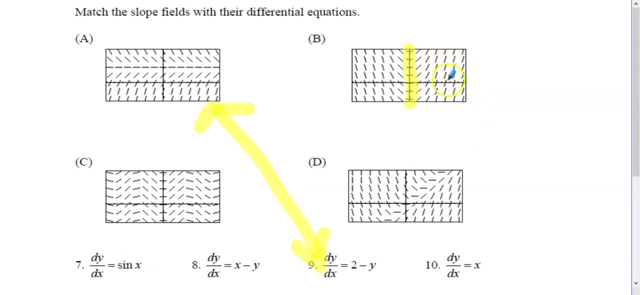 So I'm not guaranteed that just because when my x value is positive, my slope is positive. if this is the differential equation I'm using to build my slope, I'm not guaranteed that just because when my x value is positive, my slope is positive. 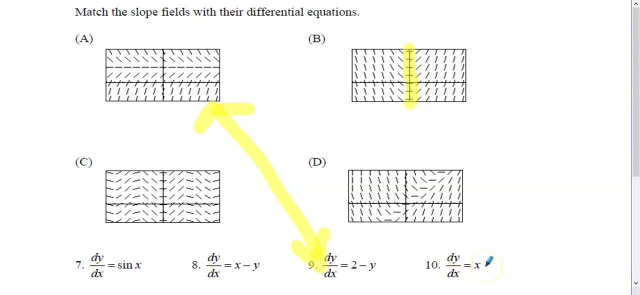 but I think for this one I am guaranteed to have that happen. Let's look at a little bit more information, since this one was a little bit more of a narrowing down process than that first one was: Look at all these slopes over here. 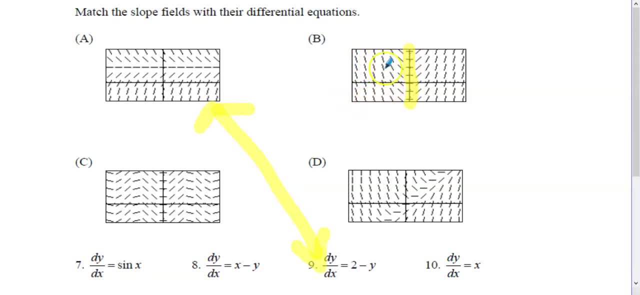 It looks like if x is negative, my slope has to be negative. All of these slope segments here are negatively sloped. This has that property. If x is negative, the value of this derivative is clearly negative. If x is negative here, well, if I do sine of. 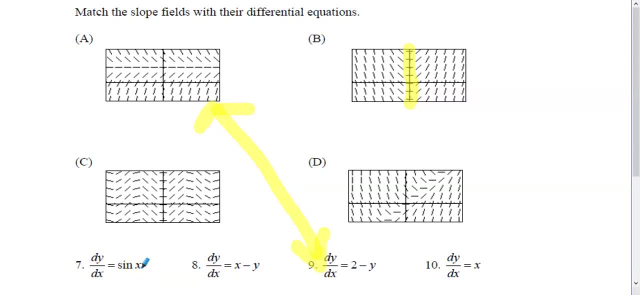 negative pi by 2, I get negative 1.. But if I do sine of negative 3, pi by 2, that's positive 1.. So this isn't always going to be negative. if x is negative, but this one is, 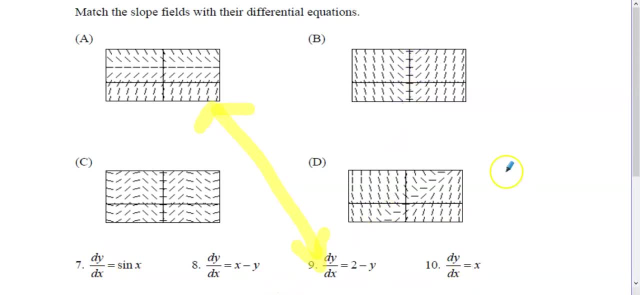 And that's pretty much the clincher here. so we'll get rid of that and we will match up slope field B with differential equation number 10.. So now we'll move on to these two at the bottom. So number 7, or, excuse me, with slope field C. 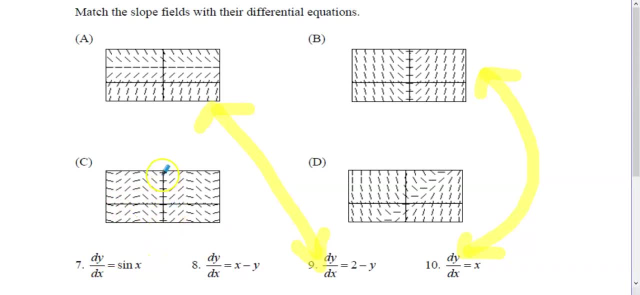 and we've kind of already done the analysis here- We have the zero slope on the x-axis or, excuse me, on the y-axis again. So when x is equal to zero, we have zero slope. This has that property. We just said that a few minutes back. 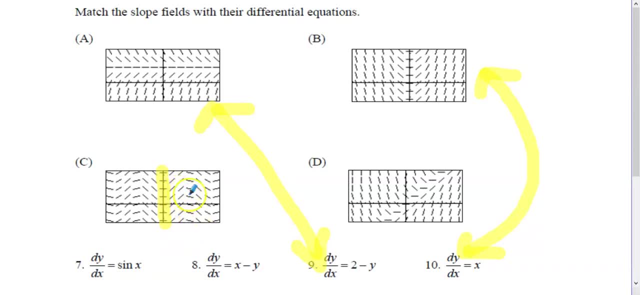 We see that sometimes in the first quadrant we have positive slopes, but sometimes we have negative slopes. We argued that that's what's going to happen with this. Sometimes, when x is positive, sine of x is positive. Sometimes, when x is positive, sine of x is negative. 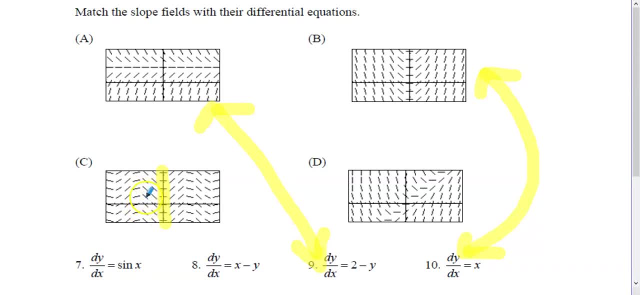 When x is negative, sometimes the slope is negative, sometimes the slope is positive. This is definitely going to match up with slope field C. And then the final one. just through process of elimination, we know what the answer is right. These are going to have to go together. 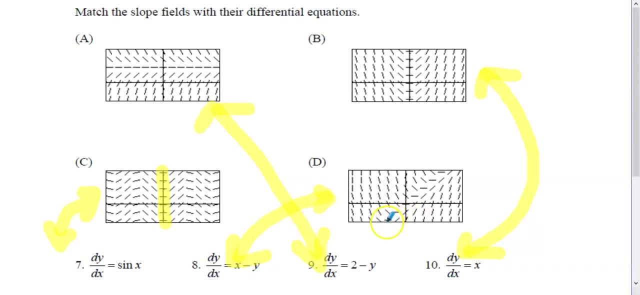 but let's try to look for some evidence to confirm why. So look at where those zero slopes are. for this one They're down this diagonal. So what's true about that diagonal? Well, it looks like zero zeros on that diagonal. It looks like one, one, two, two. 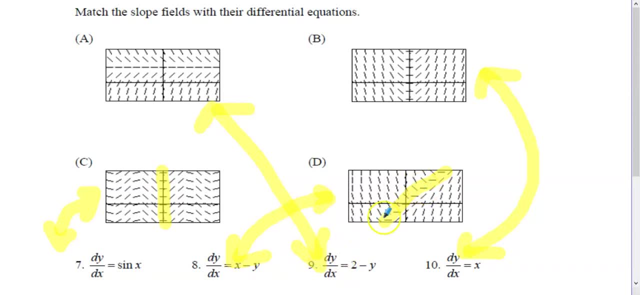 So it looks like one minus one. Yeah, that gives me zero slope. Two minus two: Yeah, that gives me zero slope. Three minus three. four minus four. Negative one minus negative one. Yeah, all of those are going to work. 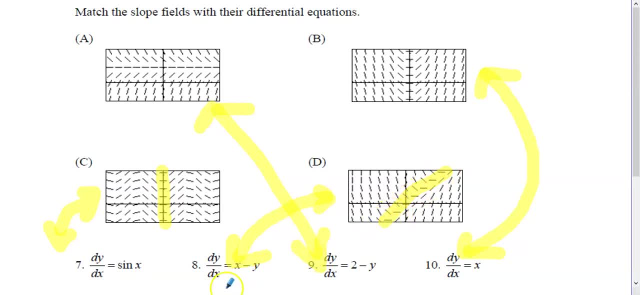 So it looks like the zero slopes do correspond, at these ordered pairs, to when this differential equation is going to equal zero. We can look for other information if we had to narrow it down further. Look for some positive slopes, negative slopes. In this case we matched it up a little bit more quickly.